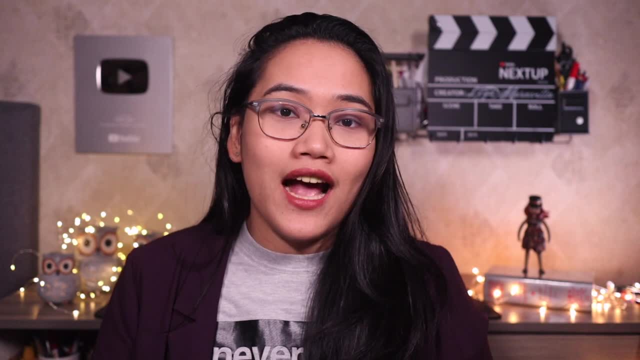 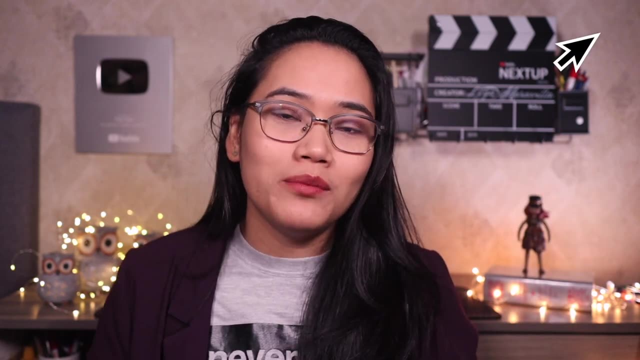 If you want to learn more about that- how you can be a channel sponsor, how can you be a rookie, a member or an MVP- click right here on the i button for more information As well as the perks that you can get if you become part of the team. 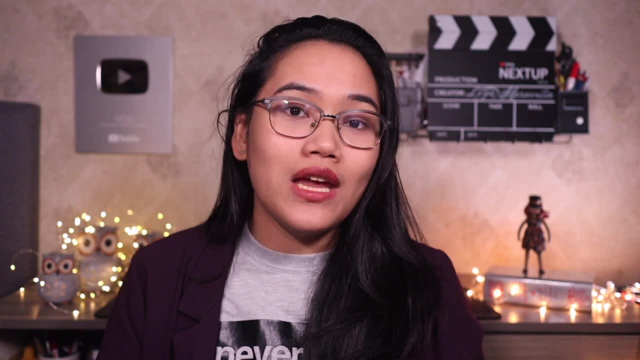 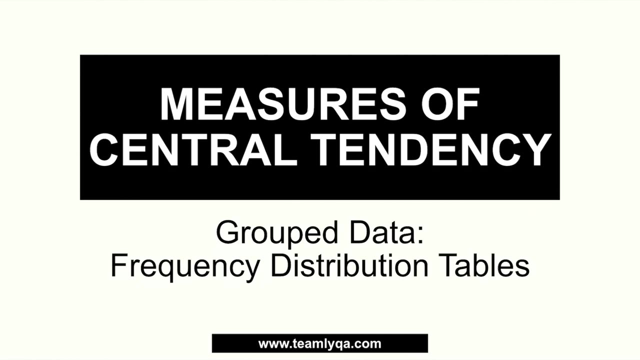 So thank you so much to all of you, And now that we have that out of the way, I'm going to jump into our discussion today. I'll see you in a bit, Okay, so this time we're going to talk about making frequency distribution tables. 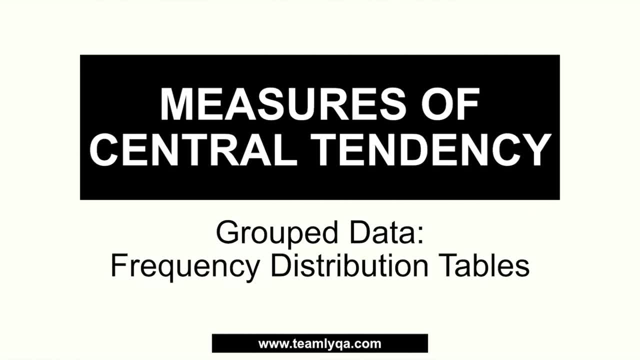 Again, we're going to do it piece by piece so you don't get lost. We're not going to overwhelm. We are going to talk about the things you need to consider and kung paano siya bubuoin Okay. Last time we talked about how to get yung mean, median and mode ng ungrouped data. 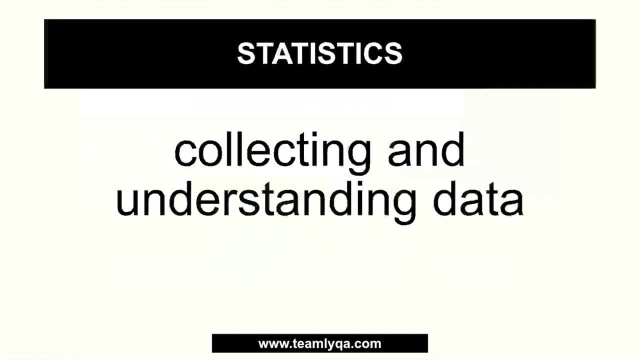 Pero ngayon grouped data naman, And anong ibig sabihin niya? Now a quick review lang. We talked about how statistics is all about collecting and understanding data. Again, it's an oversimplification, but it's fairly accurate. 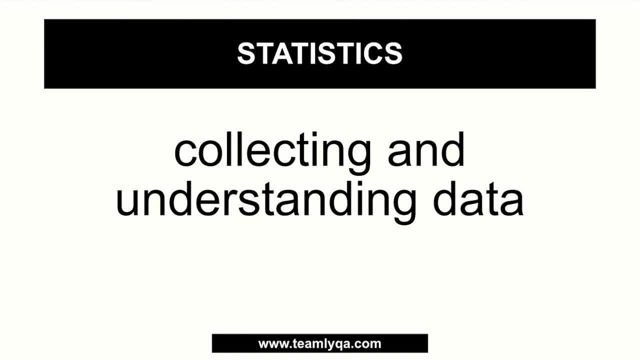 Ang goal natin is to collect data And make sure na we make some sense of it, Okay, At syempre maging accurate din yung pagkakabasa natin. Now, nung kinuha natin yung mean, median and mode last time, ito yung data set natin. 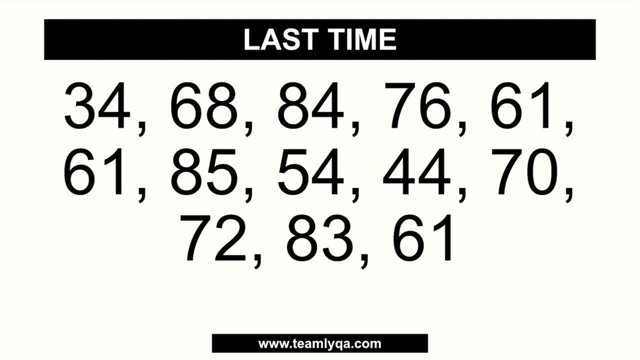 So kung titingnan natin kaunti lang, sila Fifteen numbers lang yung pinag-uusapan. Or kung ito ay study, fifteen lang yung participants nung study na yon, Pero that's rarely the case. 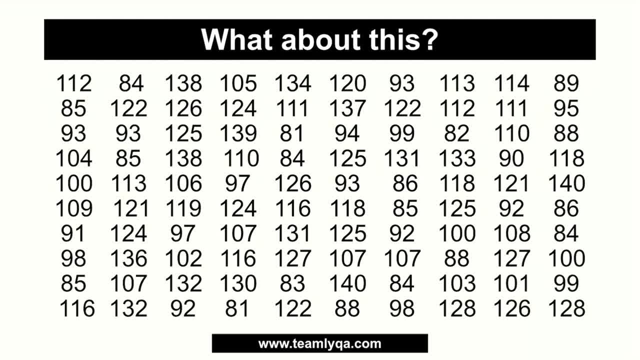 Usually it's more Okay: In order for a study to be valid Or to be kahit pa paano mas reasonable, dapat marami talaga, or malaki yung iyong number ng participants. So paano, kung ganito na siya karami. 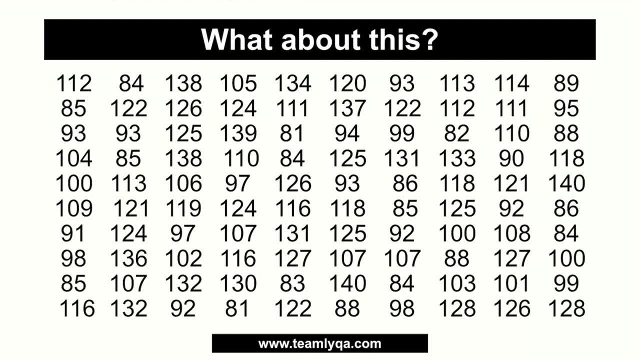 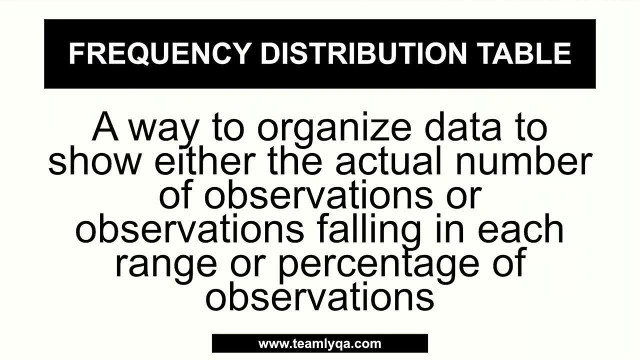 How do we deal with this type of information? Doon na pumapasok yung grouping ng data. Okay, Now how do we do that? We are going to talk about yung frequency distribution table. This is a way to organize data to show either the actual number of observations 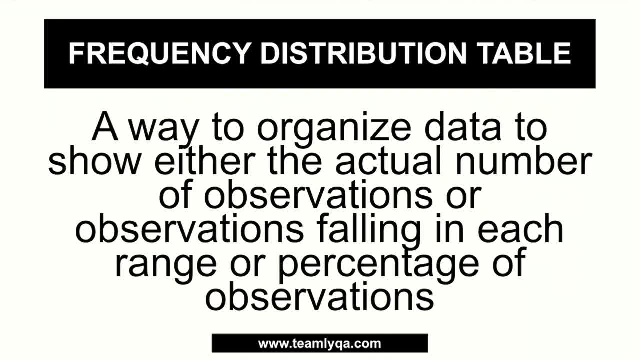 or observations falling in each range or percentage of observations Sa case natin. okay, we are going to use it to classify yung iba-ibang mga range ng data into different classes. Okay, Now pagsabing frequency distribution. ibig sabihin, ima-mark mo kung ilang beses siya lumabas. 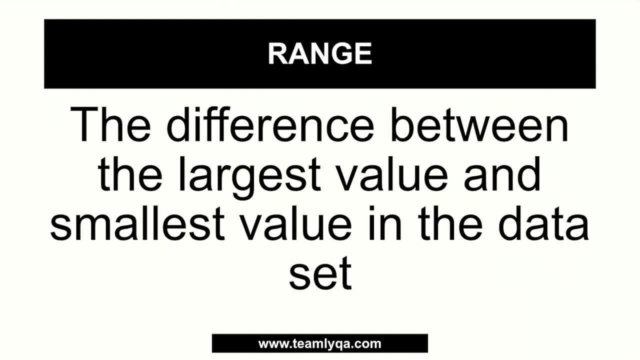 Na kung maliit yung data size mo, okay lang, Pero kung yung range mo ay malaki, dapat i-break down na natin siya into smaller pieces. Na ano ba yung range? Ang range is the difference between the largest value and smallest value. 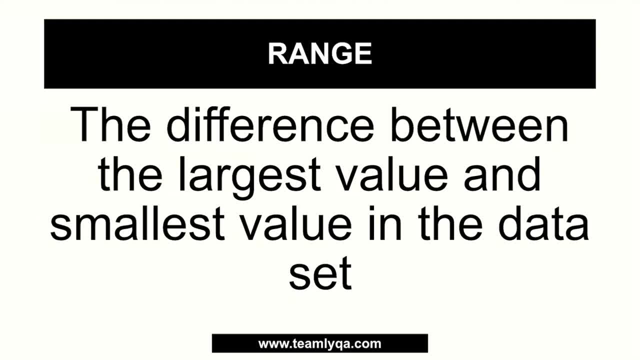 Ang range is the difference between the largest value and smallest value in the data set. So paano natin siya kukunin Ang pinakasimpleng paraan, kukunin mo lang yung pinakamalaking number. 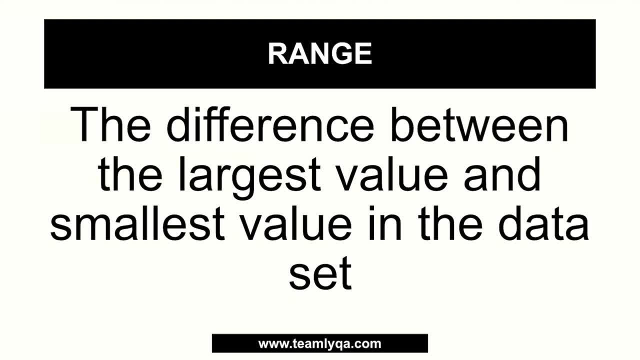 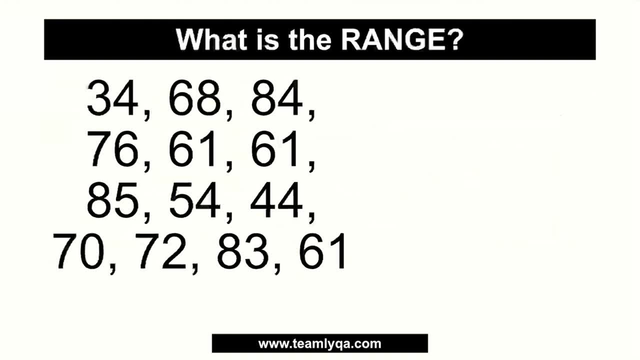 Kukunin mo yung pinakamalita number, Isusubtract mo yung pinakamalit sa pinakamalaki at makukuha mo yung range. So if we have this, yung original set natin ng information, ang range nya would be: kukunin natin yung pinakamalaking number, 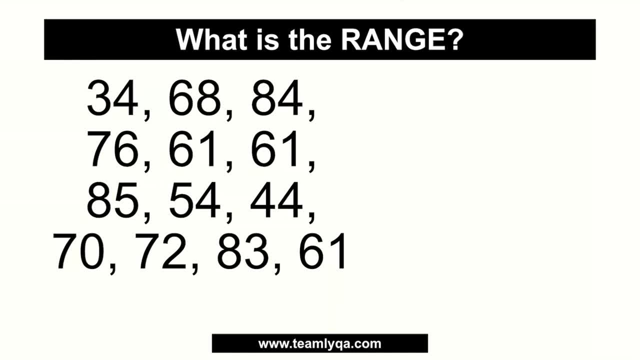 Okay, that would be 85.. So yung 85.. Tapos, isusubtract natin yung pinakamalit naman na number. In this case that would be 34.. So 85 minus 34, this is going to give us 51.. 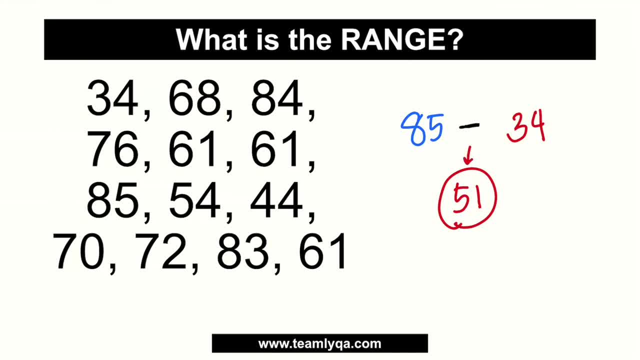 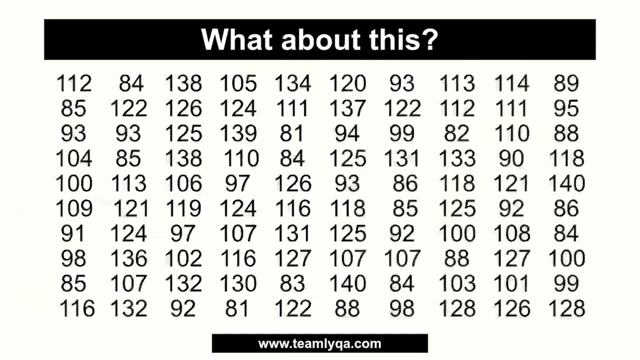 So 51 yung range ng set ng numbers na ito. Okay, So again, it's the biggest number minus the smallest number. Now, if we have something like this, ano naman ang kanyang range. And why does it matter? 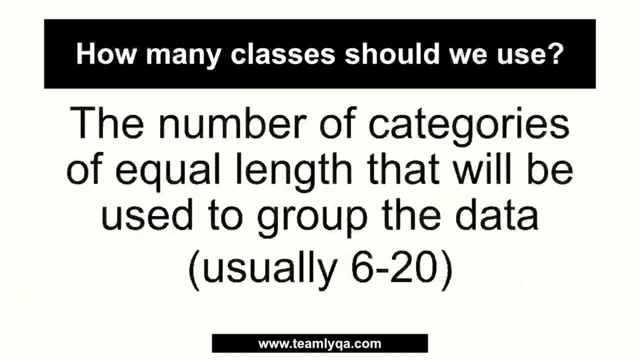 Kasi this will help us determine kung ilan yung classes na gagamitin natin doon sa paghahati natin sa ating table. Now, ano yung classes, Now the classes. ang ibig sabihin nya is the number of categories of equal lengths that will be used to group the data. 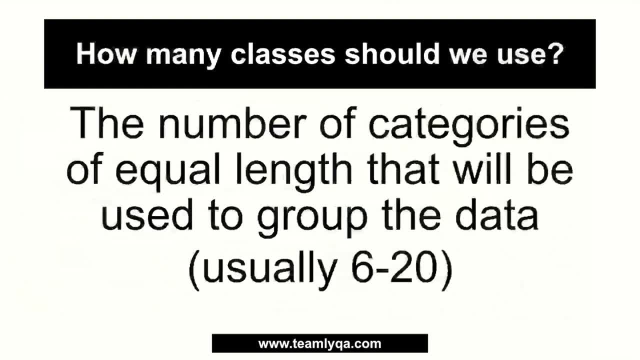 Ibig sabihin again, it has to be a specific number of categories, Tapos dapat equal yung lengths, Or minsan tinatawag rin siyang width ng category. Ano ibig sabihin doon? 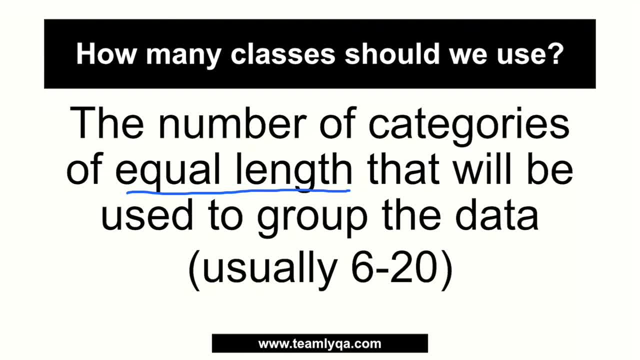 Dapat. yung range ng bawat isang class ay pare-pareho, siya dapat. And usually yung classes nasa range siya ng 6 to 20 classes. Now, kung medyo na-confuse kayo dun sa mga terms na yan, papakita natin kung paano siya gamitin. 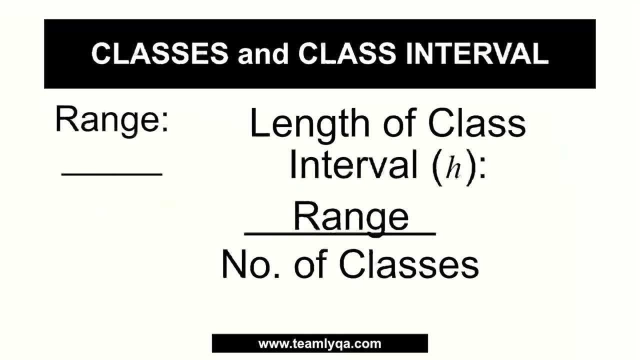 Again yung meron tayong classes and class interval. Ang idea is kukunin mo muna yung range, So again it's the biggest number minus the smallest number. Tapos to get yung length of class interval mo. 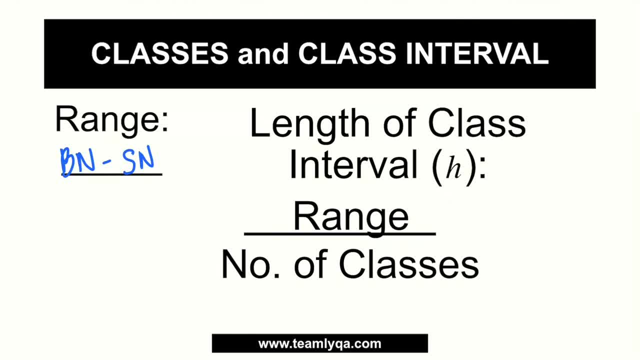 kukunin mo yung range tapos i-divide mo siya sa kung ilan yung number of classes na gusto mong ipakita doon sa iyong table. Now, how do we decide that? Let's take yung ating giant set ng numbers na ito. 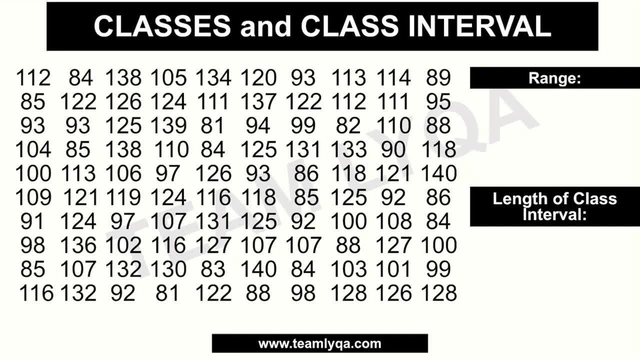 So ang dami nito we have this is 10 by 10, tama ba O 10 by 10.. So ibig sabihin 100 numbers, yung nandyan. Kukunin muna natin yung range niya. 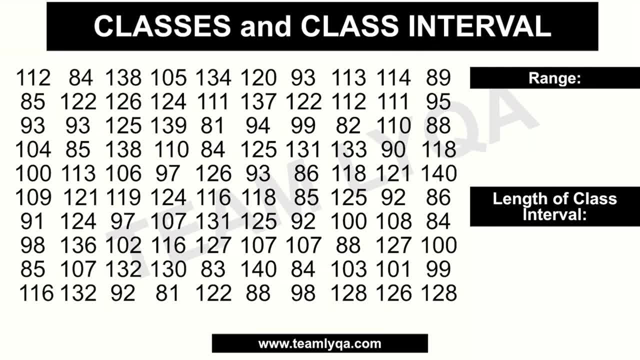 So how do we get that? We get the biggest number, So biggest number minus the smallest number. Now, hahanapin na natin yung dalawa ngayon, So biggest muna tayo. So meron tayong mga line of 2, 120,, 127, 130.. 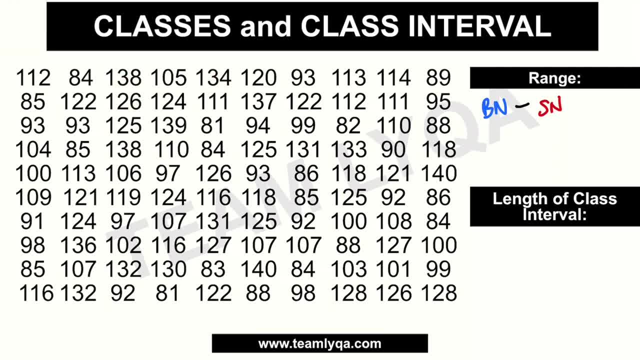 Meron pa bang 140?? And dito na pumapasok yung kapag nasa stat po tayo dapat may attention to detail tayo. So ang ating candidate would be 138.. Hanap pa tayo kung may mas malaki pa sa 138.. 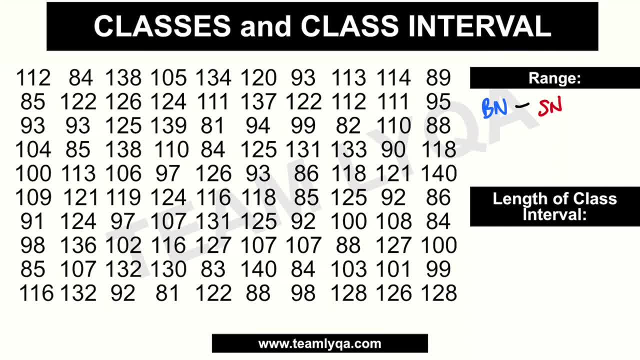 May 139?. Okay, So ito siya Meron bang 140? Tingnan natin, O yun 140.. Okay, So again, kaya very important to pay attention, Mataas ba sa 140? Wala. 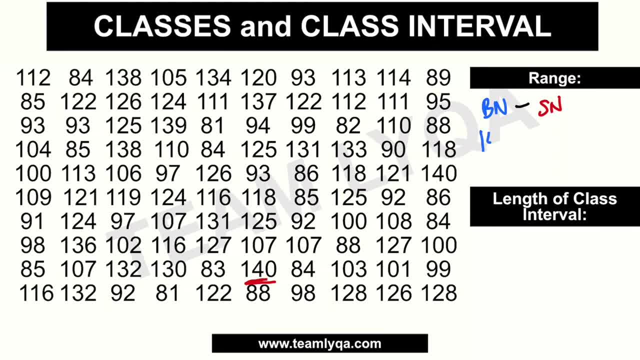 So ibig sabihin the biggest number here would be 140.. So isusubtract natin sa kanya yung smallest number, naman Hanapin natin yung pinakamaliit. So dito meron tayong mga line of 8.. 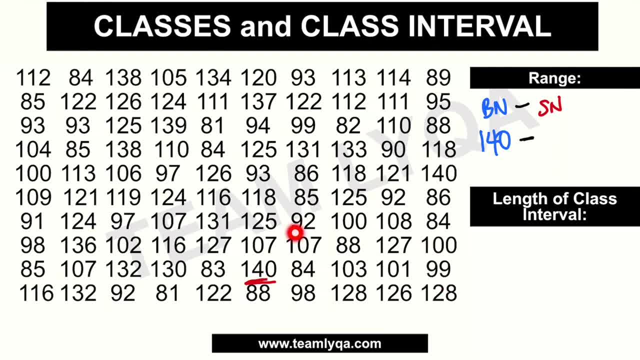 Walang line of 7, no. So pero meron tayong 81. Ang tanong: meron bang 80?? Tingnan natin kung may 80. Okay, wala, So the smallest number is 81.. 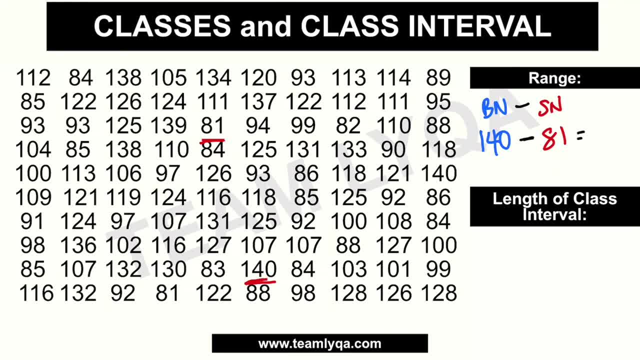 So isusubtract muna natin sila, So 140 minus 81, that would be 59. So the range is 59. Now, kung ang range natin ay 59,, so mga around 60 siya. 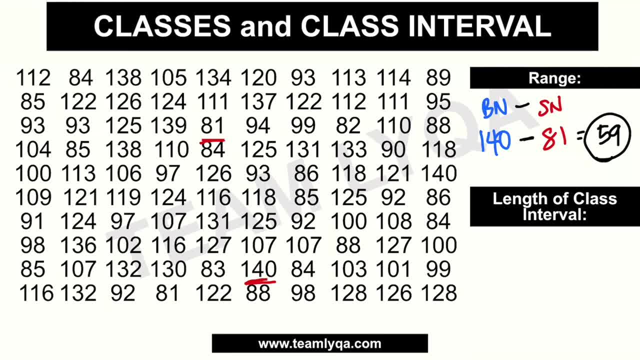 pwede tayo mag-decide on class interval Now. kung pwede natin siyang hatiin sa 6. Kunyari, Okay. So kung meron akong 6 na classes dito, ang magiging length of class interval ko would be. 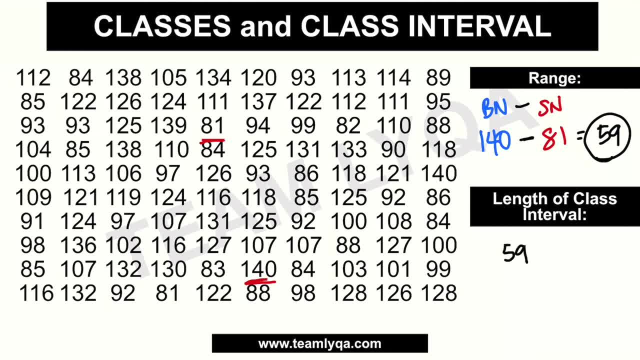 I will take the range, which is 59,, tapos i-divide ko siya sa 6.. Okay, That way parang nasa ang length or class width na tinatawag would be about 9 point something. 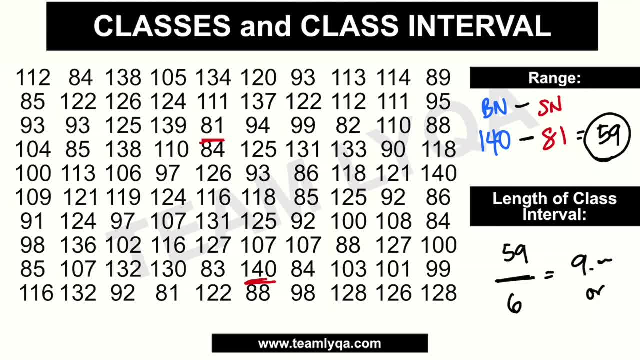 Okay, Or i-round up na lang natin siya, and always dapat naka-round up yan, i-round natin sa 10.. Okay, So ibig sabihin nun, bawat hati ay mahati sa tig, sa sampung number sa loob ng bawat class. 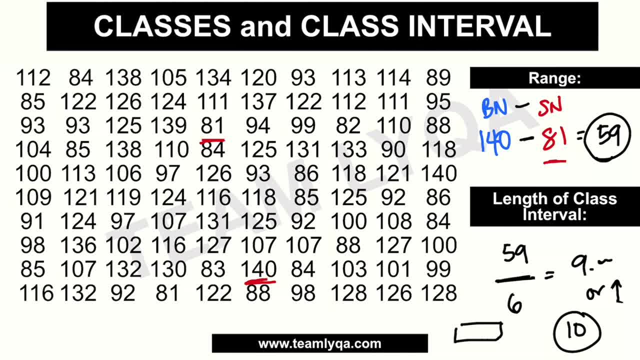 Now ano yung sampung number na yun: 81 to 90,, 91 to 100, hanggang umabot siya dun sa limit, Hanggang umabot siya dun sa limit natin na 140.. Okay. 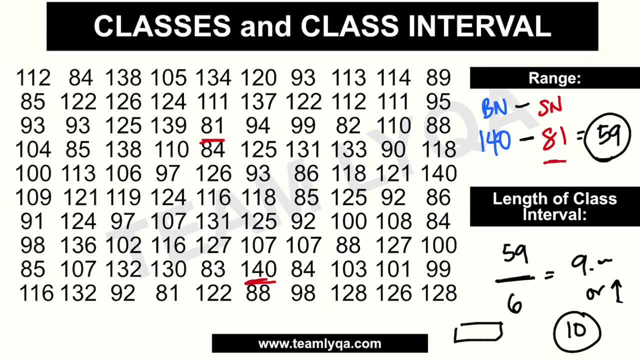 So, after you have that, kung ilan na yung classes again- in our case we decided to have 6, at kung ilan yung class interval, which is 10,, pwede na natin gawin yung table? 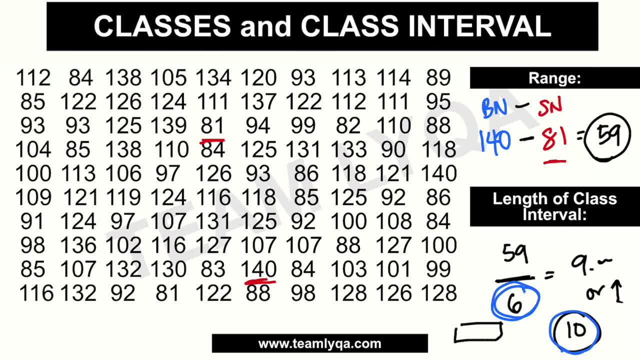 Now quick side note here. If you are doing yung work na required sa'yo ng teacher, kung modular learning man yan, or if you're back in school, you could ask them kung ilan yung required number of classes. 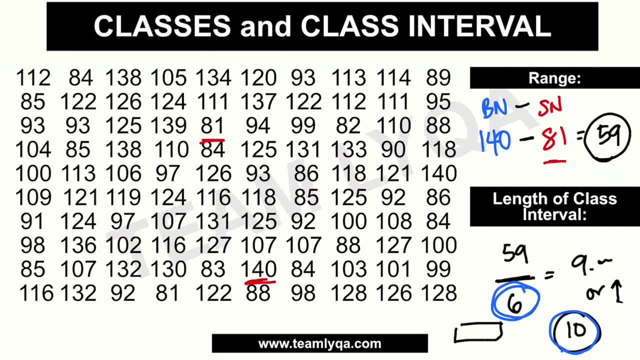 In most exercises or classes. you can ask them how many classes are required In most exercises or quizzes. sasabihin naman nila yan sa inyo, Kung hindi, naman, kung independent, yan ibig sabihin, ikaw ang pwede mag-decide, pwede ka mag-decide on your own. 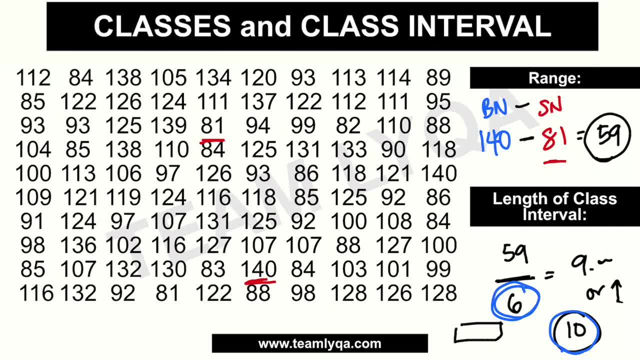 Sa akin. I usually bunch the numbers sa either interval size: siya na 5 or 10.. Kasi mas madali siya, mas visually okay siya. So I would go 51 to 55, and then 56 to 60.. 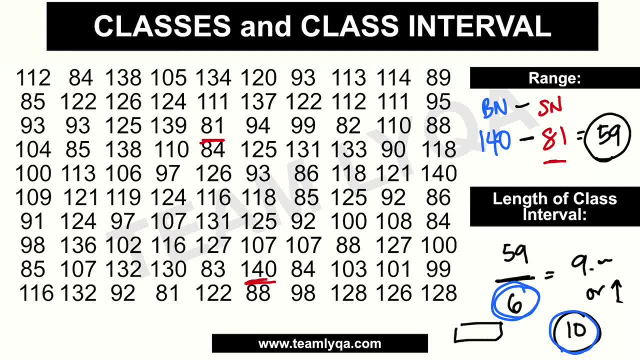 Yan, ang class size nun is 5.. Or yung gagawin natin ngayon, which is by 10.. Okay, so ito na yung ating table, tapos i-coconstruct na natin siya. 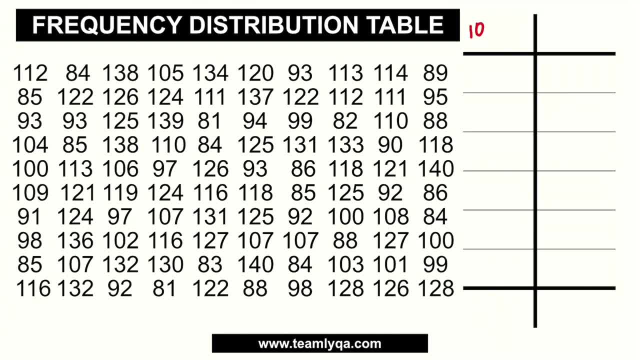 Now, if, for example, yung data ang ibig sabihin niya ay IQ scores ng participants natin, pwede natin siya i-label like that. Ilalagay lang natin yung mga range per class. So sisimulan na natin sa pinakamababa. 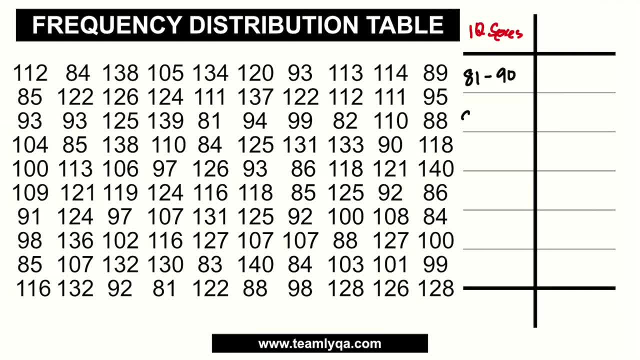 We have 81 to 90.. 91 to 100.. You have 101.. 110.. 111 to 120.. 121 to 130.. Tapos, yung pinakalast, 131 to 140.. Make sure that you double-check itong mga information na yan. 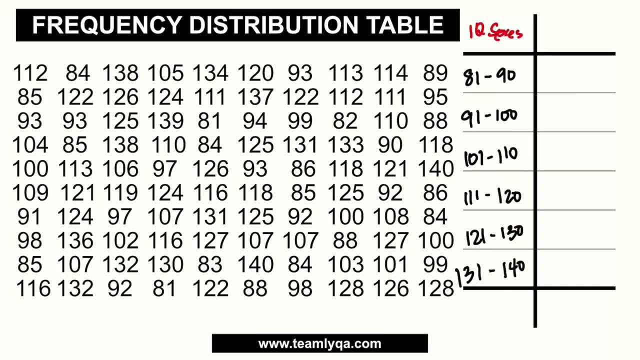 Kasi mas mahirap magkamali tapos babalikan mo pa later. Next, gagawin na natin yung frequency. Okay, so yung frequency would be kung ilan yung lalabas na within yung range ng bawat class na yan. 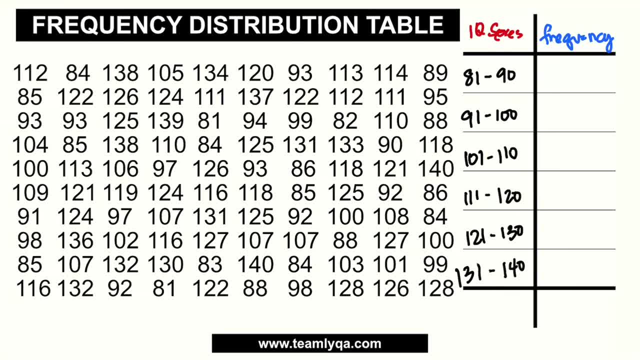 Now here's my piece of advice, Lalo na if you're dealing with a huge number ng mga elements or ng mga data, make sure that you cross out everything. Okay, Tapos, itatali natin sila. Okay, let's start. 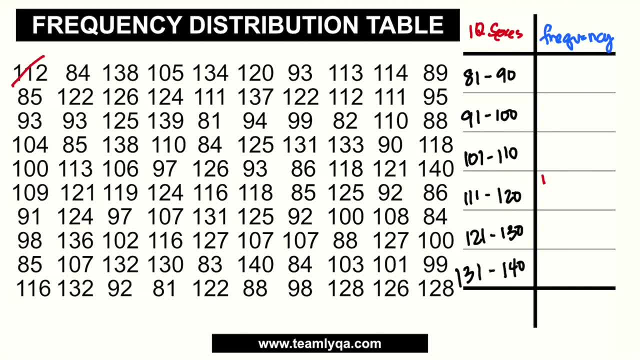 If you have 112, ilalagay natin siya dito Okay, 85 would be here. 93 is right here. 104, dito siya: 100 is here. 100 is here, Okay. 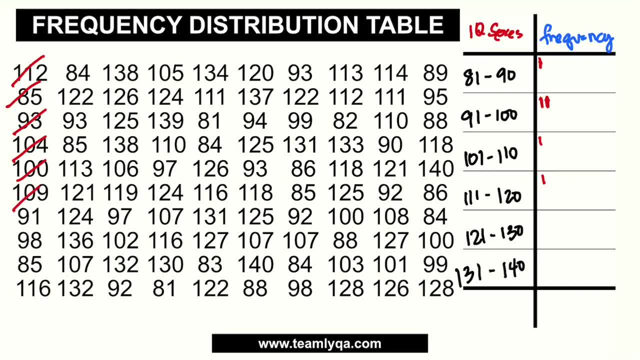 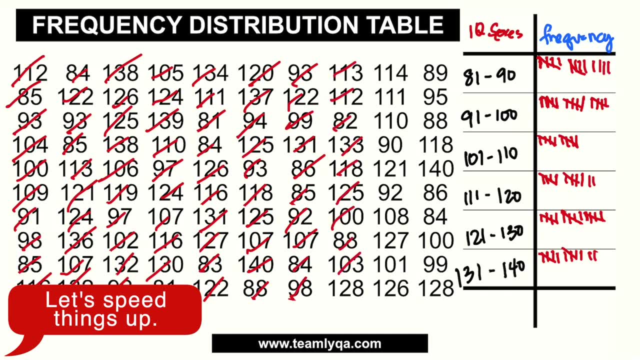 109 will be here. Okay, so natali ko na siya Ngayon, ilalagay ko na yung numerical value para ma-double check natin siya. So here we have 5, 10,, 15,, 19.. 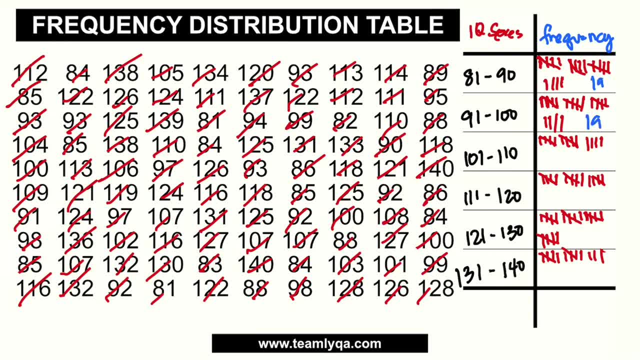 Dito 5, 10, 15,, 19 din siya. This has 14.. Ito ay 15.. Ito ay 20.. Tapos, here we have 13.. Again, pag-inadd ko lang yung 19 sa isa pang 19.. 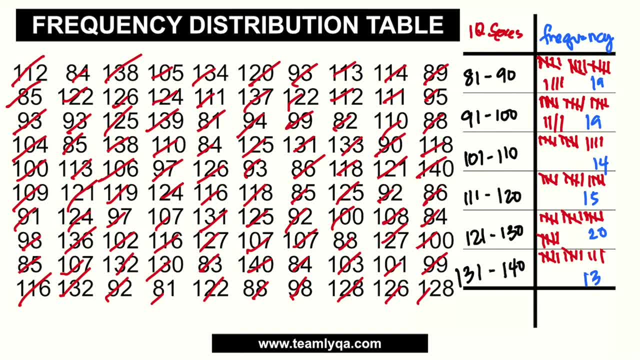 Tapos 14,, 15,, 20, and 13.. Ayan, 100 naman yung total niya. So kung ano na yung total niya, we can say na okay, na-cross out ko na lahat. 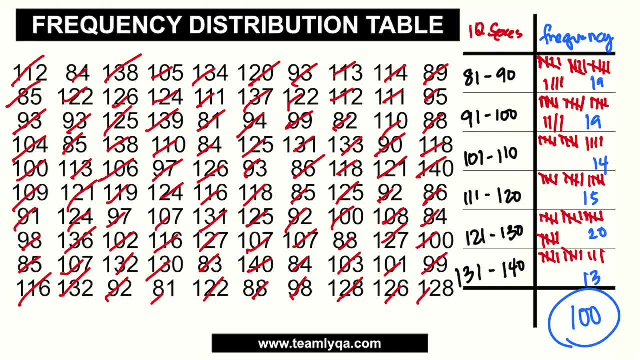 And now we're going to use itong data na ito sa mga calculation natin ng mean at iba pa Okay, In a later video. So again, ito na yung ating frequency table: 81 to 90,, 19 times siyang nag-appear or 90 times yung frequency niya. 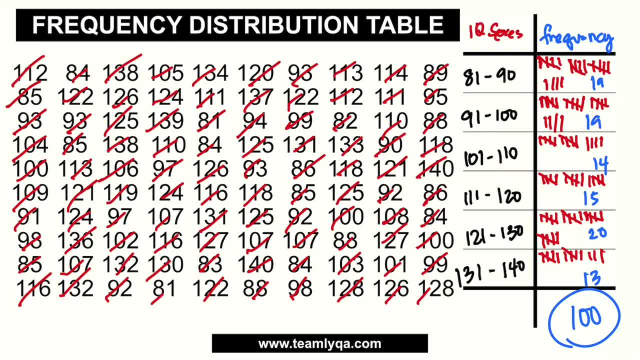 91 to 100,, 19.. 101 to 110.. 14,, 15,, 20, and 13.. Now, it's very time-consuming And it's part of the process, Pero the more you do, it honestly very zen din siya. 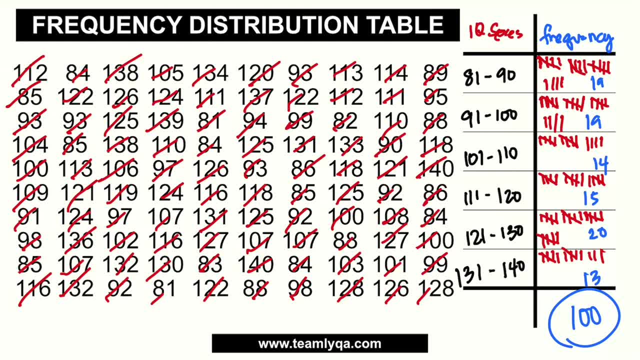 I like doing it And this is one of the things that I enjoy most about statistics. Okay, So again, ano, yung mga key takeaways natin ngayon: How to build your table, How to build your class size. 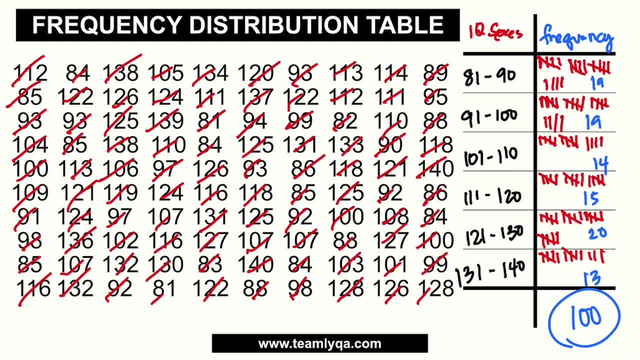 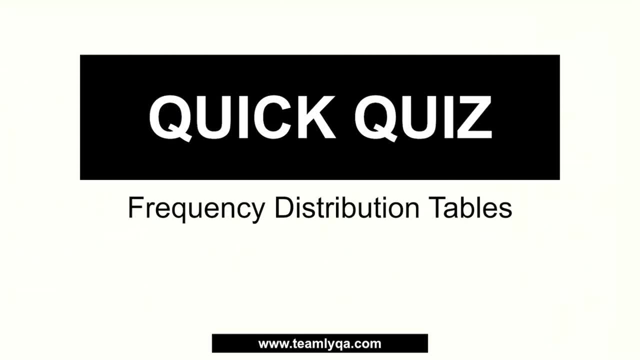 And how to construct yung frequency. Okay, Now that we have that quick quiz, muna tayo. So I'm going to give you a set of data And I want you to keep this, kasi ito rin yung gagamit natin is to solve natin next week. 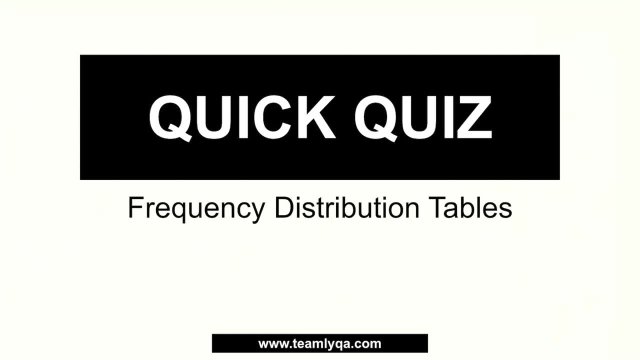 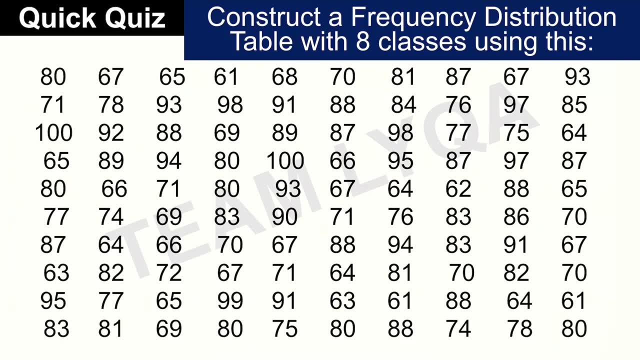 Pag kinuha na natin yung mean mode and median. Okay, And if you're ready with your pen and paper, your timer starts now And let's get to this. Okay, And in this video, I'm going to tell you how to do that. 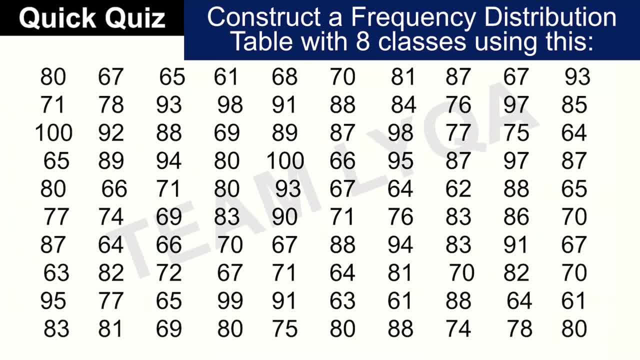 And I'm going to give you a set of these Rubik's Cube And I want you to keep your paper, And I want you to keep your paper. Okay, I just want to let you know that there are a number of things that I love about this. 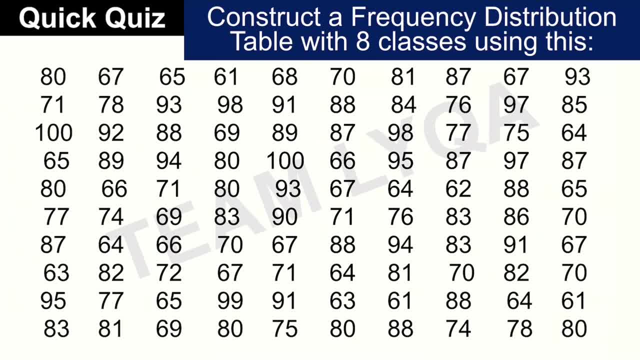 paper. So in this video I'm going to show you a few things about this paper from my talk show called A Canine- in a Minute- And part of the talk show is going to be about that- And I'm going to show you what's in the book. 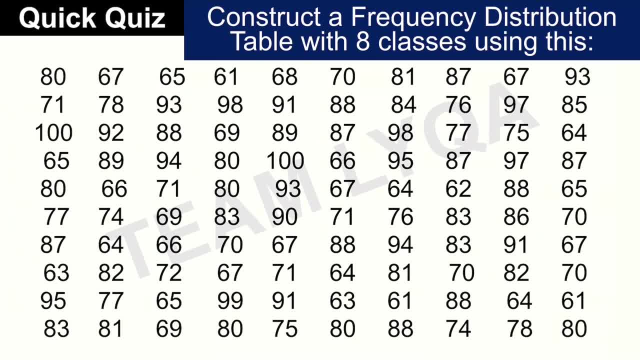 And part of the talk show is going to be about the book in a minute, So please be sure to watch until the end of today's video, And I'm going to show you the whole paper before I come back. Thank you, Thank you. 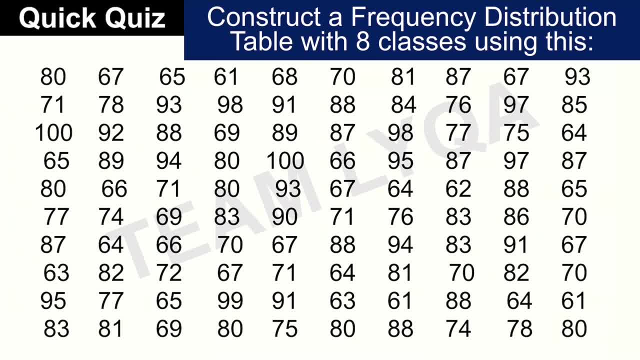 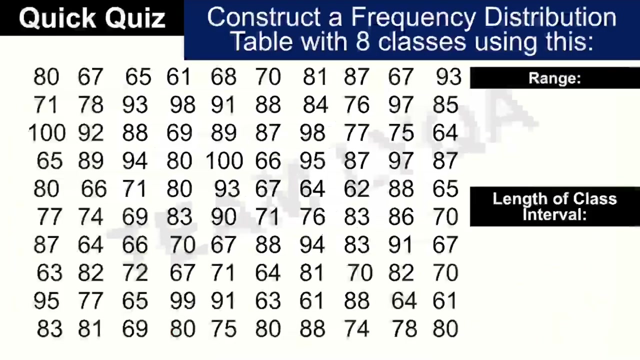 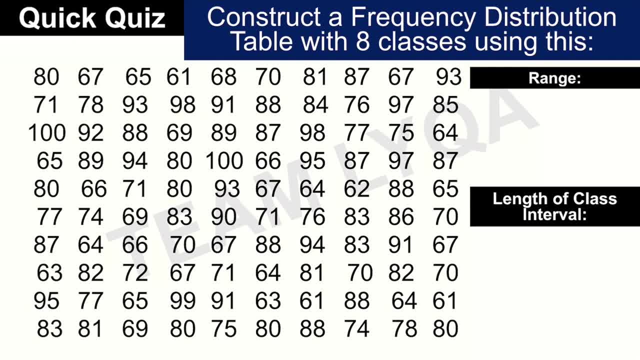 So let's look for the biggest number. Okay, it has 100.. Is there a bigger one here? No, there's not. So that's our biggest number. That would be 100.. Then let's minus the smallest number. 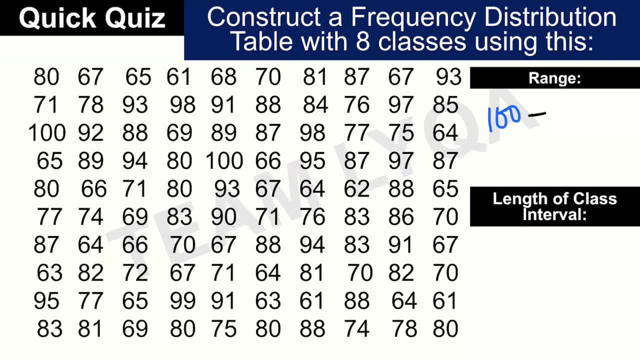 The smallest number. does it have 9 of 6?? Yes, So that would be Okay- 61.. Does it have 60?? Let's see if there's 60.. Okay, there's none, There's only 60.. 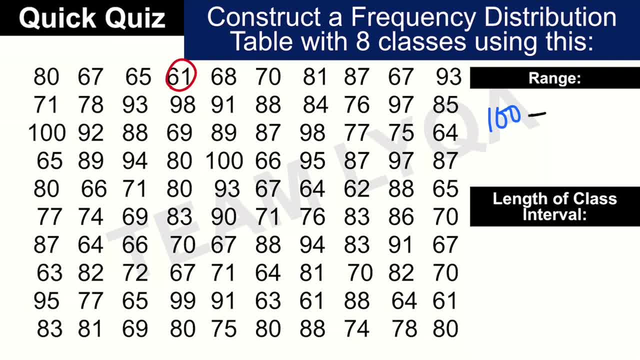 So the smallest number is 61. So its range is 39. Now let's say: And it's given 8 classes, So it means This 39, let's divide it by 8.. Okay, so what will come out of it would be a little over 4, almost 5.. 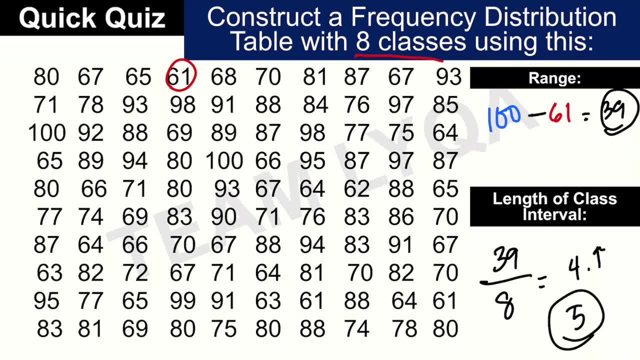 So it means The length or width of our class interval would be 5.. Okay, so that would be 61,, 62,, 63,, 64,, 65.. Then 66 to 70.. Okay so, let's construct the table. 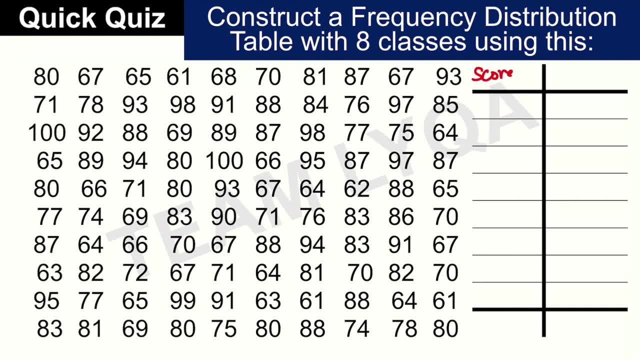 Okay. so if this is its scores, let's just put each class again. Let's start with 61 to 65.. 66 to 70.. Then 71 to 75,, 76 to 80,, 81 to 85,, and then 86 to 90,, 91 to 95,, then 96 to 100. 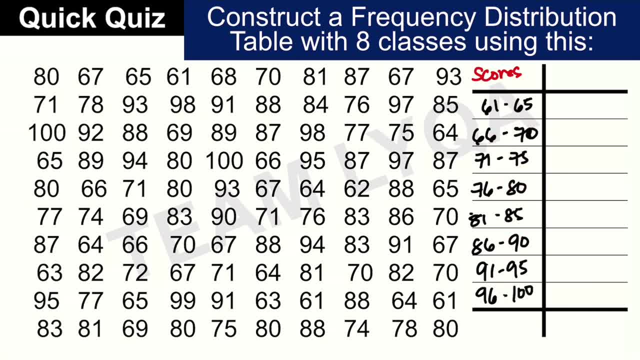 Okay, so did we miss anything? None. Okay, let's go to the frequency. So if you need to go to our time earlier, you can hit pause Again. we can review this, But I'll just solve this with you. 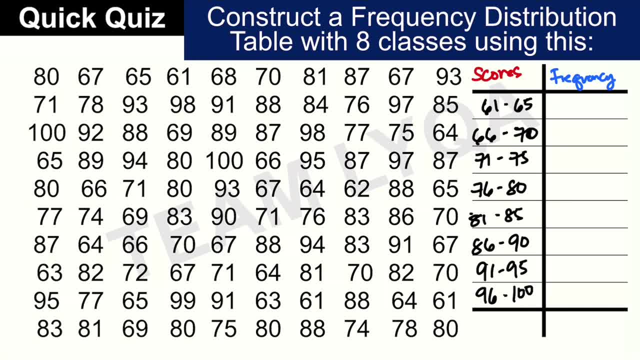 I'll speed up later, Just so we can arrive at the right calculation. Again, it's all about attention to detail, So let's put them one by one. We have 80 here, So that would be right here. 71.. 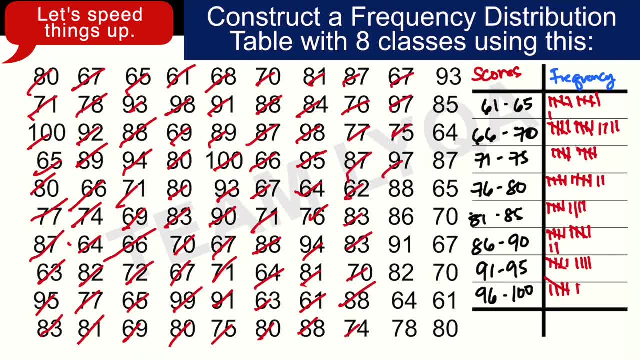 okay, so yung last ay 80. so 80 would be here and we're done again. i uh sum up lang natin yung mga tadi natin. tas i check natin kung 100 siya. so sa 61 to 65 we had 15. next here we have 17: 10. this is 14. 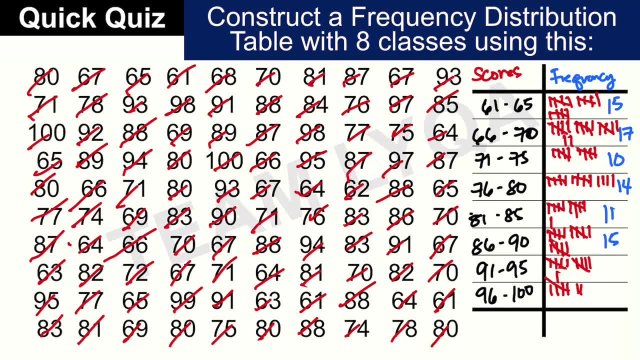 11 tapos 15. this is 11 din tapos 7. okay, so check natin. kung pag in add ko sila lahat ay 100, ba sila kasi, kung hindi siya 100, uulitin natin lahat. so yun yung pinaka. 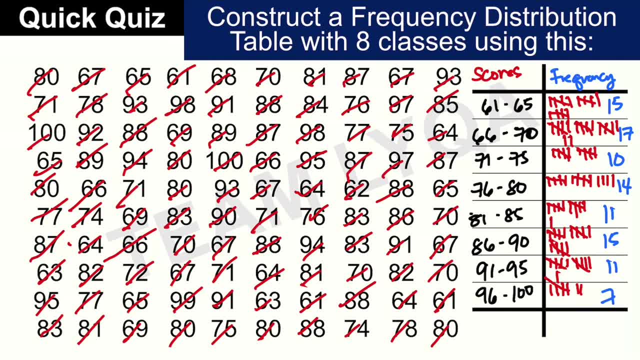 tedious na part ng statistics, kasi pag nagkamali ka ng isang beses, mali na lahat. so you really have to be careful. okay yan, so 100 naman yung total nyan we're good. okay, okay, so sana, nakuha nyo rin ito ng tama. so again we have 15, 17, 10, 14, 11, 15. 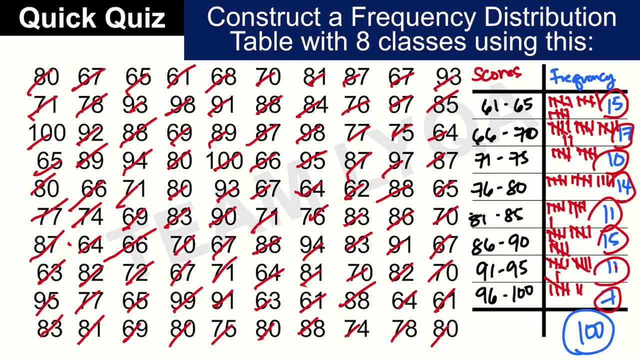 11 and then 7, tas ito yung ating mga range ng scores. okay, so now that we have that again, pag-uusapan natin kung paano kunin yung mga ibang parts, yung measures of central tendency, paano kung grouped yung data like this: keep your paper, kasi yan din yung gagamitin nating. 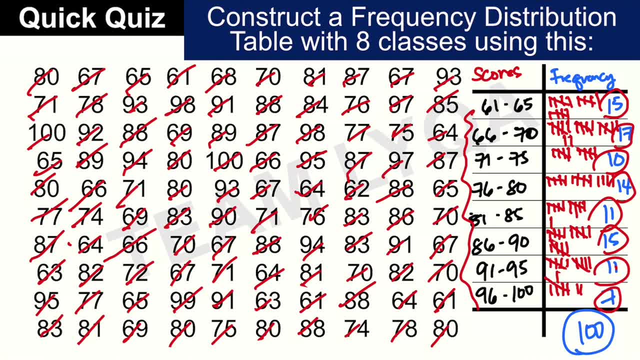 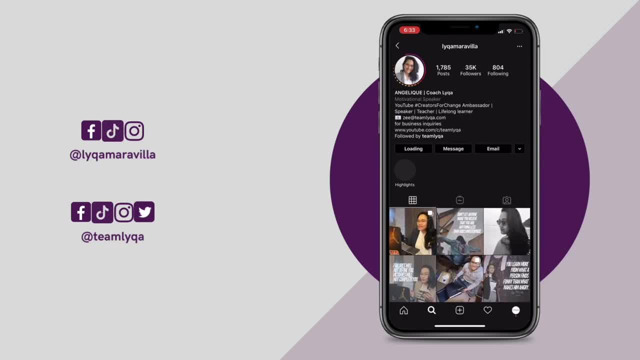 information for next week. okay, so yan muna for next week. now, if you have any questions, requests or anything, you can comment din sa baba, and if you want to make use of our quick quiz functions sa instagram, don't forget to follow me there. it's at laika maravilla. on instagram. you can check out yung mga stories doon. doon natin. 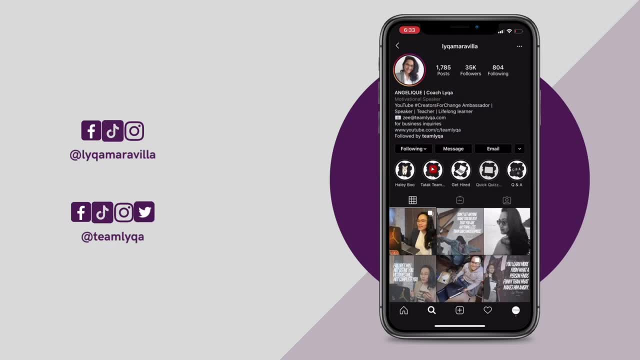 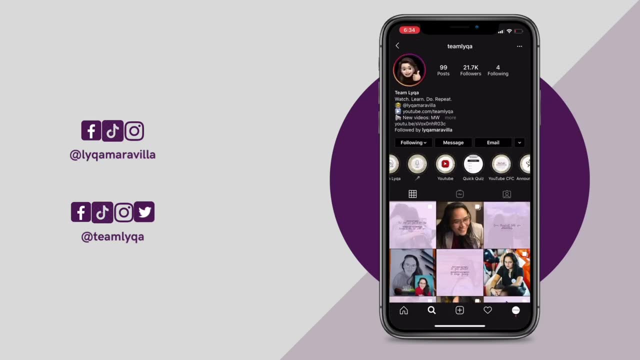 pinupost yung mga bagong quick quiz and at team laika naman for the other content: mga throwback questions, other videos na relevant sa inyo, mga nirequest ninyo at yung mga iba pang mga important announcements. okay, and if you're on tiktok you can follow me. i have two.